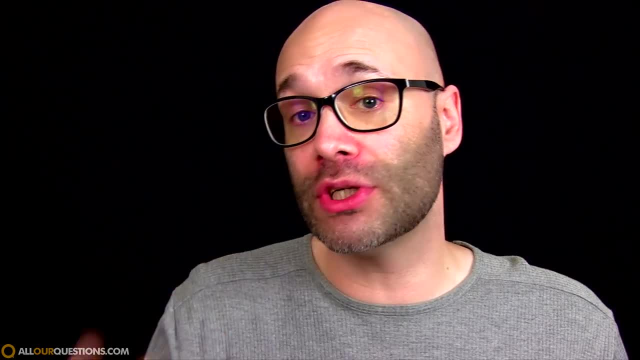 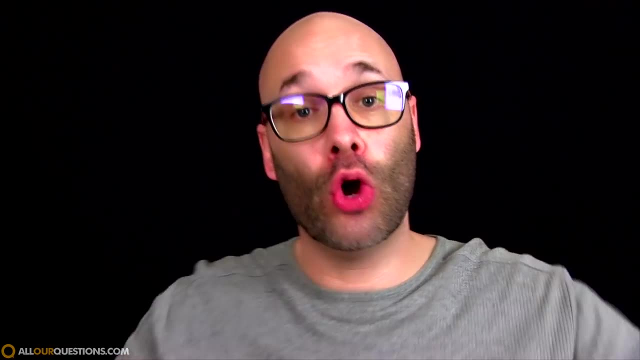 a survey where they found 42% of males and 30% of females have the same favorite color. That color is blue, And real quick, let me know in the comments down below what your favorite color is. Mine's: red. Blue evokes feelings of calmness and serenity, and it's used by 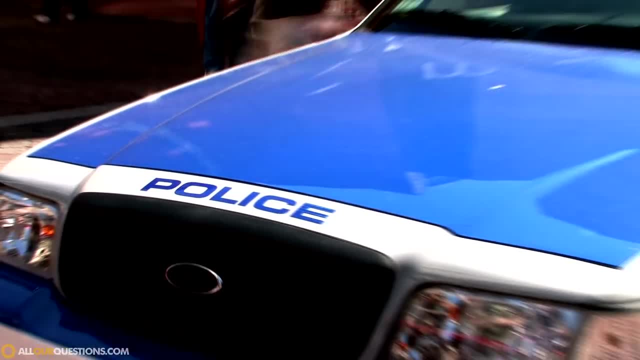 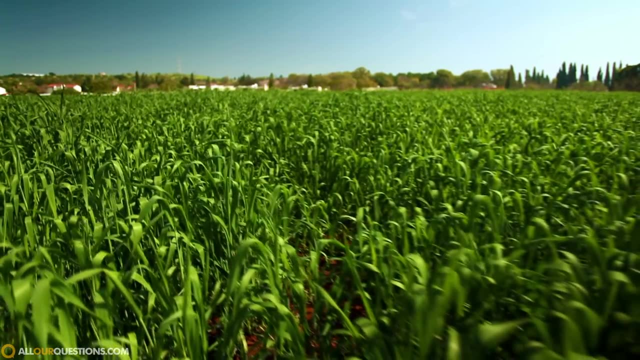 businesses and marketing campaigns, to project stability, and it's also used to project authority. Green is the easiest color on the eyes and it's symbolic of nature. Like blue, it produces feelings of calmness and relaxation. Purple is associated with royalty, wealth. 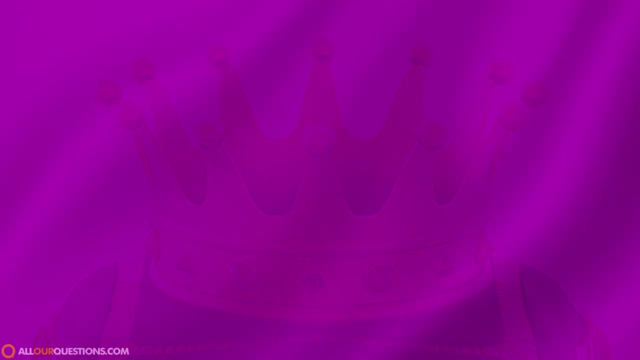 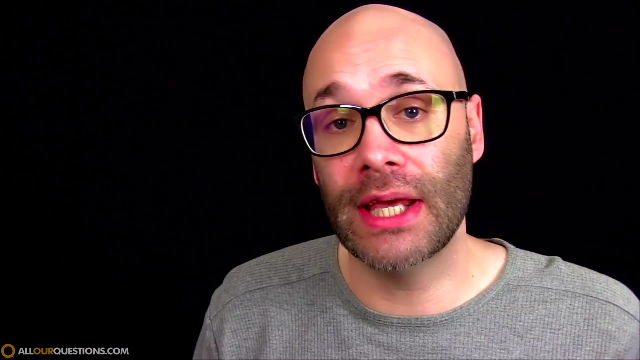 luxury and sophistication. These associations stem from the time consuming and expensive process involved in making the color purple a long time ago. Basically, they made the dye from sea snails and it was such a time-consuming and expensive process that only royalty could afford to actually. 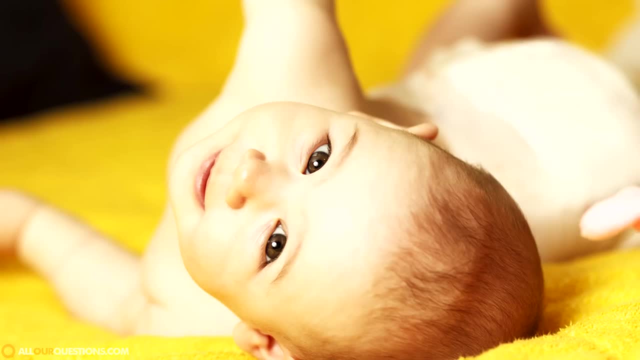 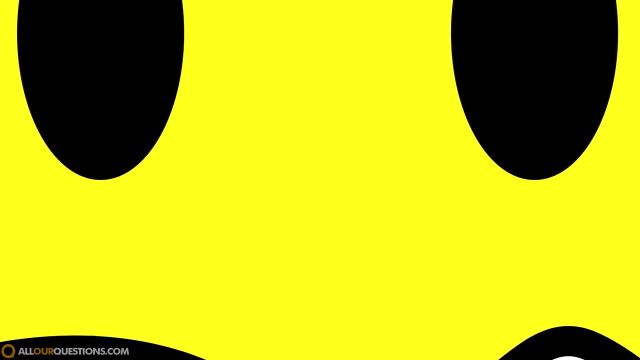 make it happen. Yellow, like red, is an attention-getter. If you have a baby, it's important that you, It's important to know that your baby will most likely cry more if it's in a yellow room. If you have a temper, you're more likely to lose it if you're hanging out in the yellow room. yellow also speeds up metabolism. 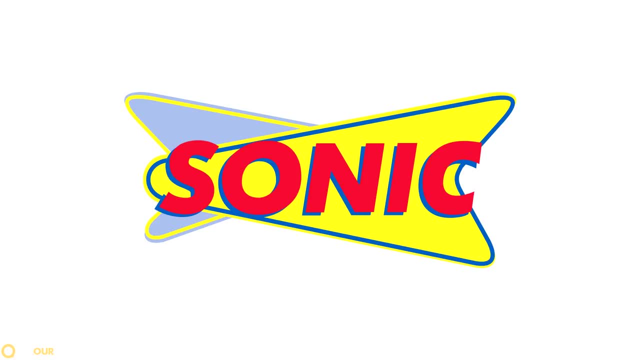 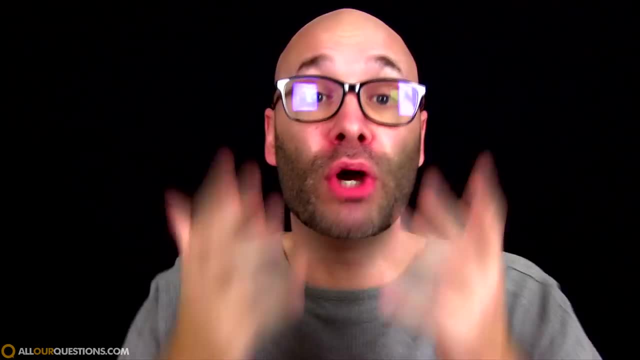 It helps us focus and it makes us hungry. think of that next time you're looking around at fast-food logos. Black is primarily associated with authority and power, as well as evil and death, But you fashion folks out there know that black can also make us appear thinner, and wearing black can also make us feel more. 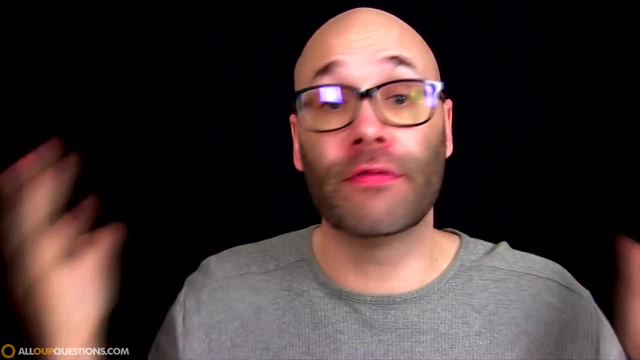 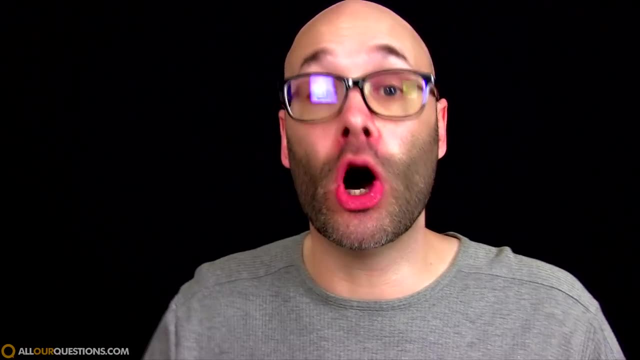 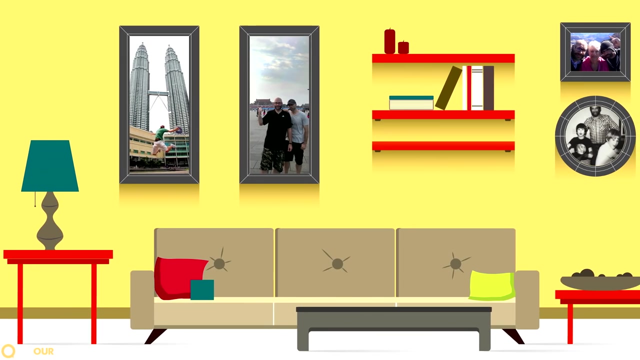 confident and Empowered. while the effects all of these colors have on us can come from Associations or instincts that are buried deep inside of our brains, Personal experience can also have a huge impact on how we perceive color. For example, if you have a lot of fond memories of hanging out in your grandma's yellow living room. 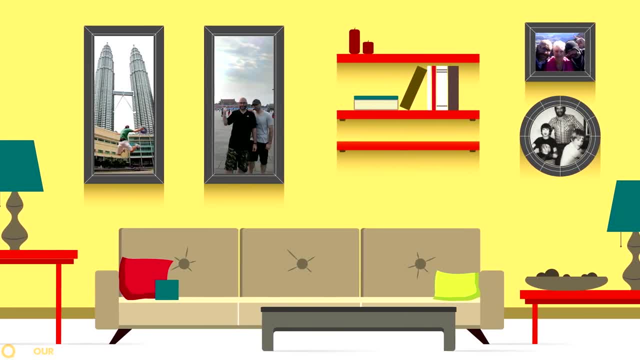 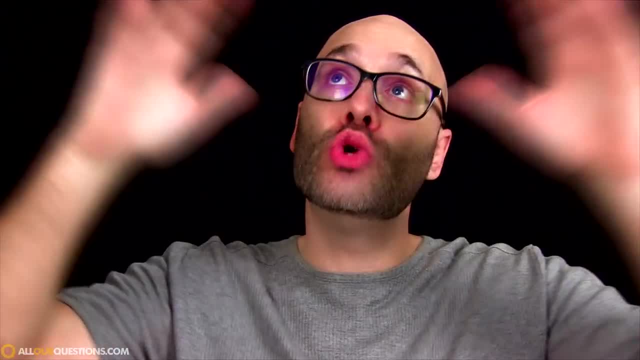 Then there's a really good chance that when you see the color yellow, Your brain is going to release some dopamine and you're gonna feel happy when you're exposed to the color yellow. now, Hopefully, you'll see this huge world of color Just a little bit differently. if you enjoyed this video, remember to give it a thumbs up. 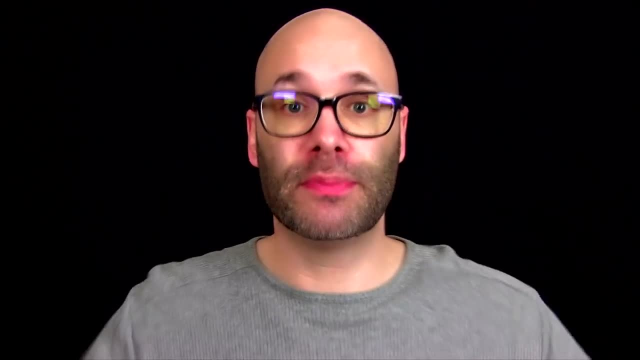 And if you're not already subscribed, make sure to hit the subscribe button somewhere on this page So you can get more answers to all our questions. Thank you so much for watching. I'll see you next time.